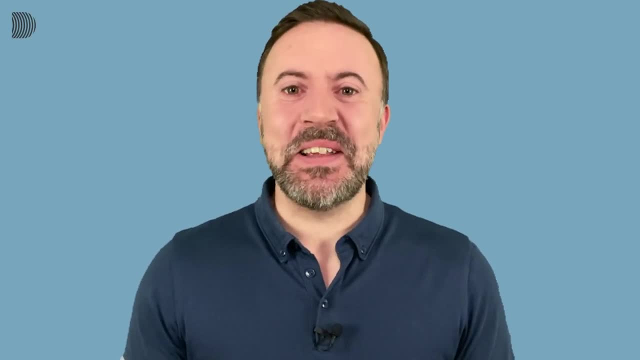 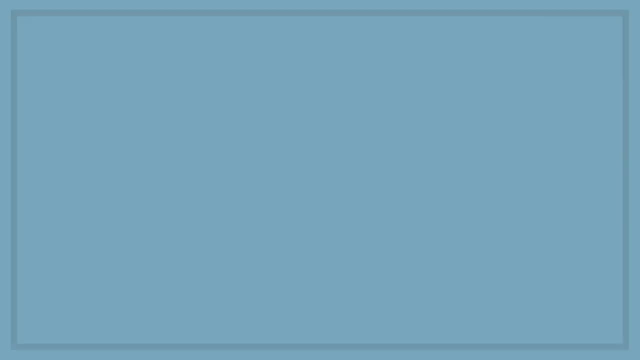 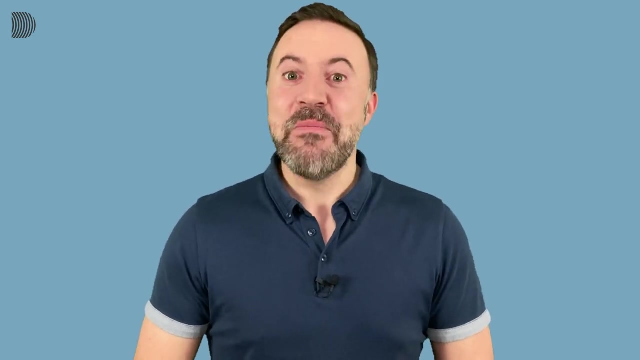 Hi everybody, Hope you're all doing well. In this lesson I'm going to show you lots of different ways to express how sure you are about things in the future. Welcome back to English for Professionals. I'm Derek and I'm here with another short lesson for you busy people. Before we get started, just a. 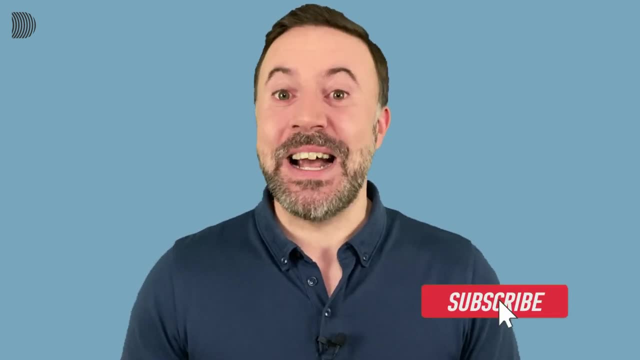 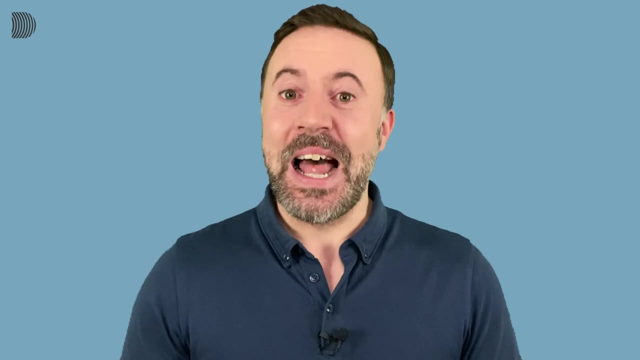 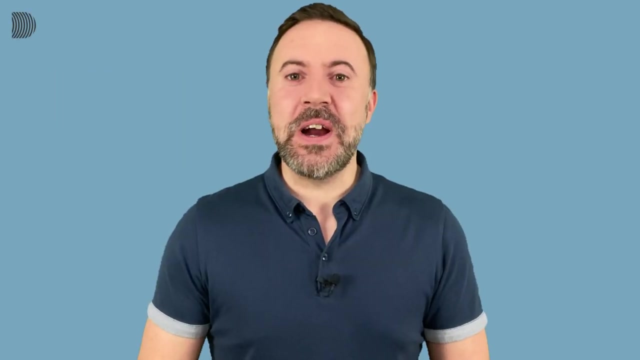 quick reminder: to subscribe to my channel, hit the red button and don't forget to click on the little bell. that way, you'll be notified every time I upload a new lesson. and now let's get started. so in this lesson we're going to look at lots of different ways to talk about. 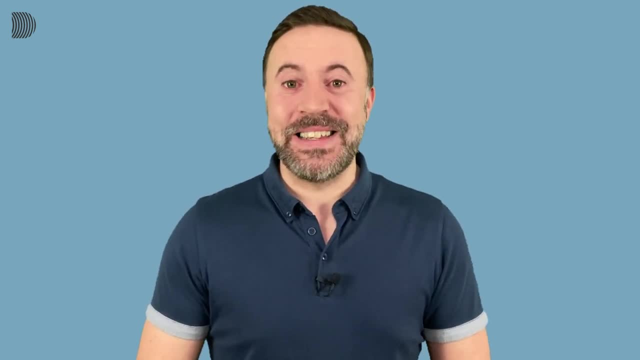 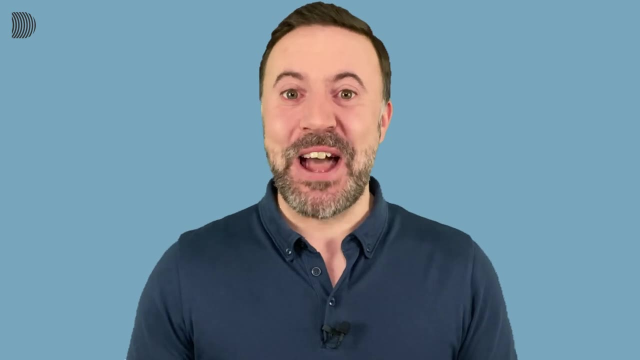 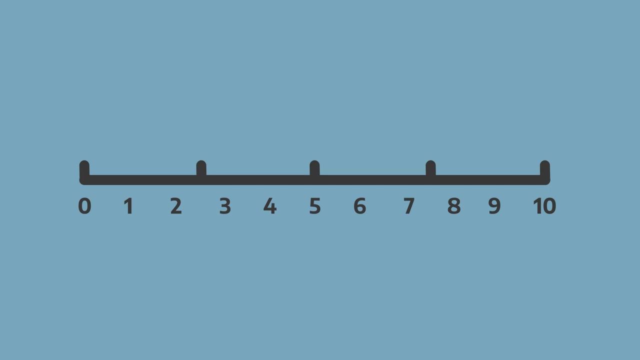 certainty, probability and possibility in the future. At the end of the lesson there's a quiz to test what you've learned. so make sure, sure you stick around for that. and now let's start by looking at this scale and some different adjectives. we'll begin at zero with impossible. impossible. then between zero and five we have. 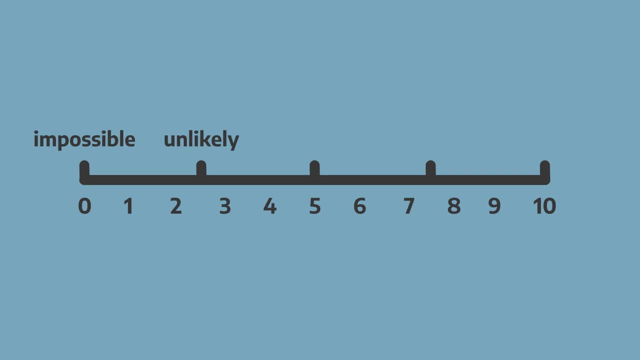 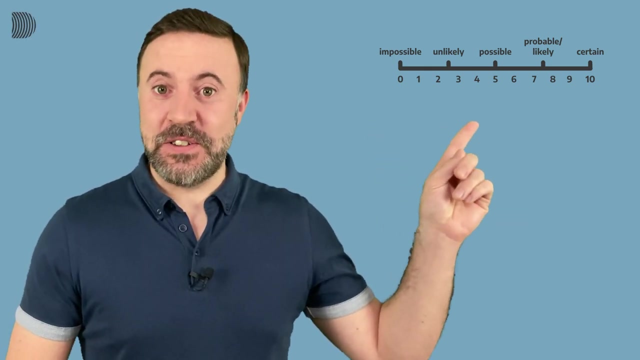 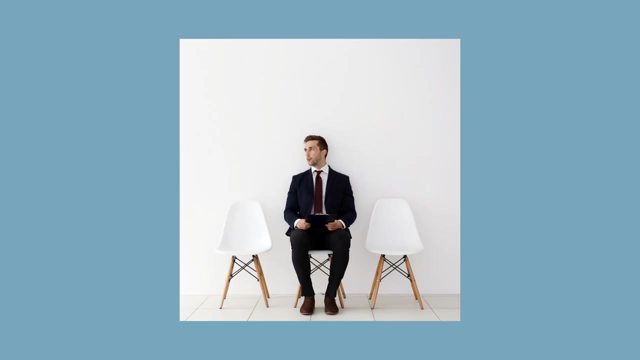 unlikely, unlikely. at five we have possible, possible, and between five and ten we have probable or likely, probable or likely, and finally, at ten, we have certain, certain. so that's our scale showing the different degrees of certainty. now let's take a look at some simple example sentences for each part of the scale. but first let's meet michael. 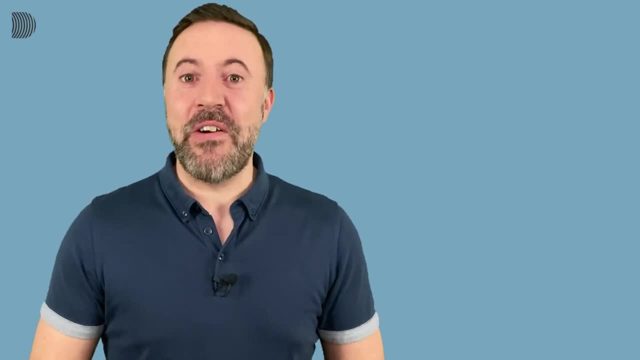 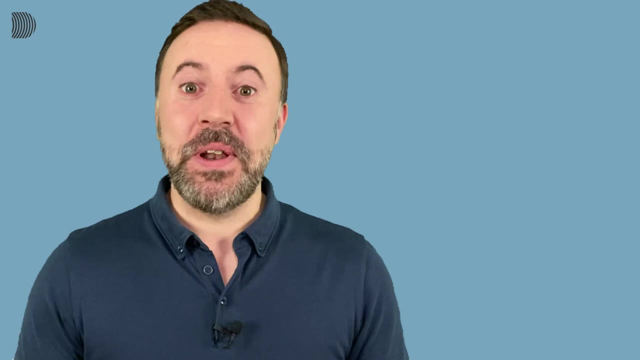 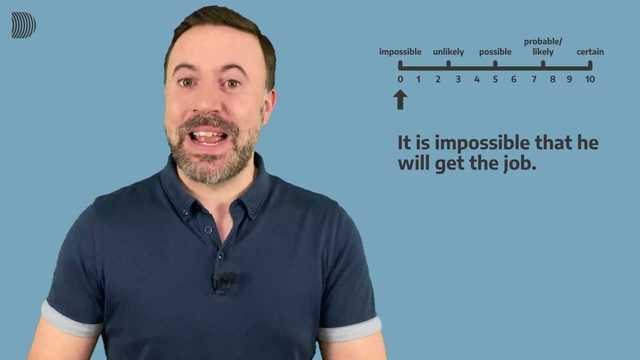 imagine michael went for a job interview, but he wasn't very well prepared, he didn't show any enthusiasm or interest in the position and he even had an argument with the interviewer. so let's start at zero and say it is impossible that he will get the job. it is impossible that he will get the job and if you want your spoken english to sound more, 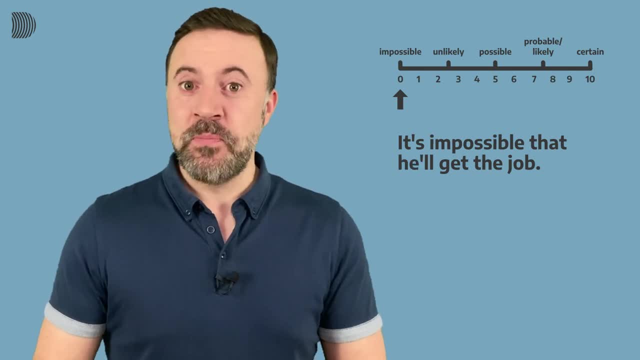 natural. we can use the shorter forms and say it's impossible that he'll get the job. say it with me: it's impossible that he'll get the job. and if you want to sound even more natural, we can leave out the word that it's impossible he'll get the job. say it with me: it's impossible he'll get the job. 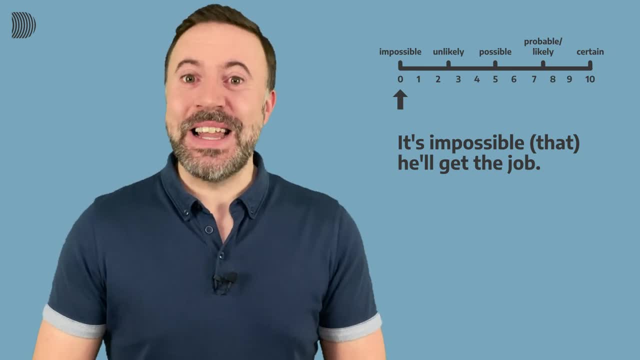 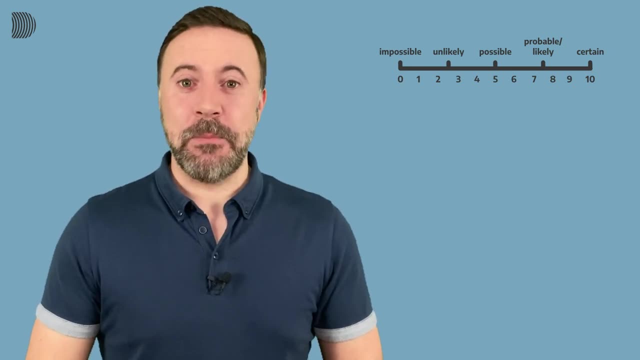 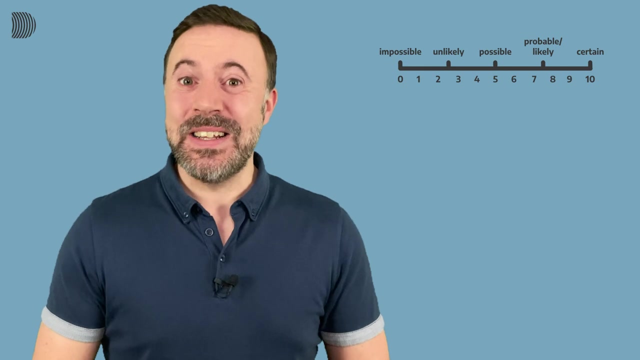 now, depending on your level, you may feel more comfortable leaving the word that in, and that's perfectly fine. now let's move on to the next part of the scale. imagine michael did do some preparation. he didn't answer the questions very well and he didn't make a good impression. so we can say: 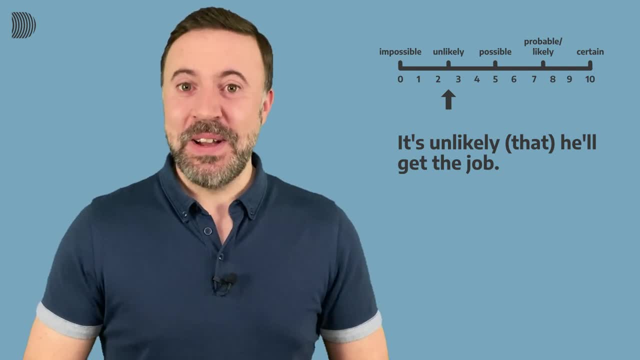 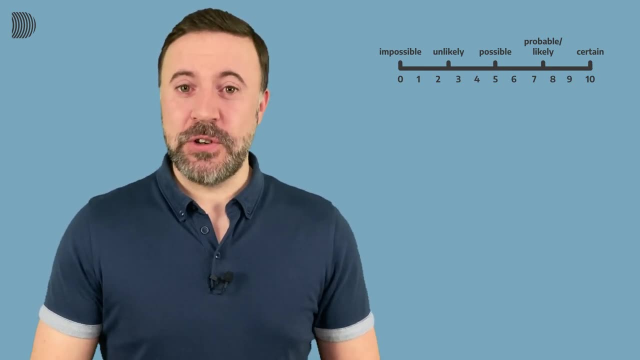 it's unlikely he'll get the job. say it with me: it's unlikely he'll get the job now. let's imagine the interview did go well, he made a good impression, but he doesn't have enough experience we can say it's possible he'll get the job. say it with me: it's possible he'll get the job for the next example. 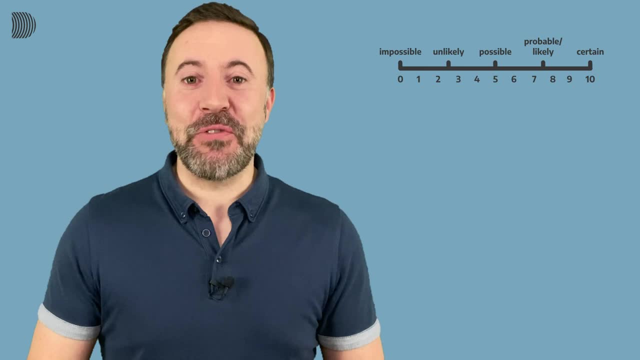 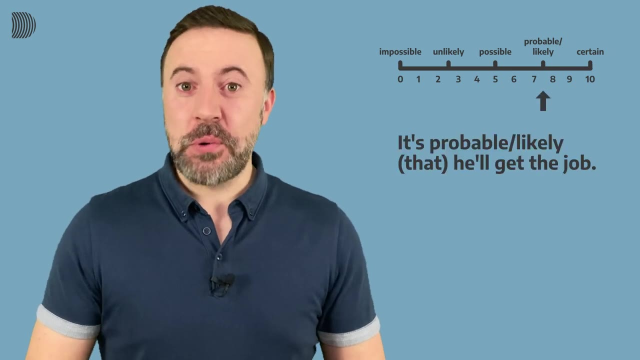 that michael made a great impression and he has more qualifications and more experience than any of the other applicants, so we can say it's probable he'll get the job. say it with me, it's probable he'll get the job. or it's likely he'll get the job. say it with me, it's likely he'll get. 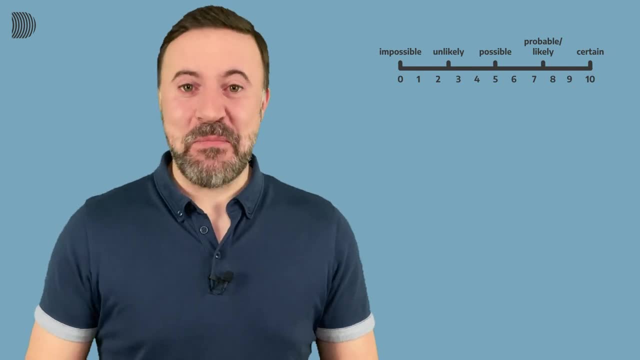 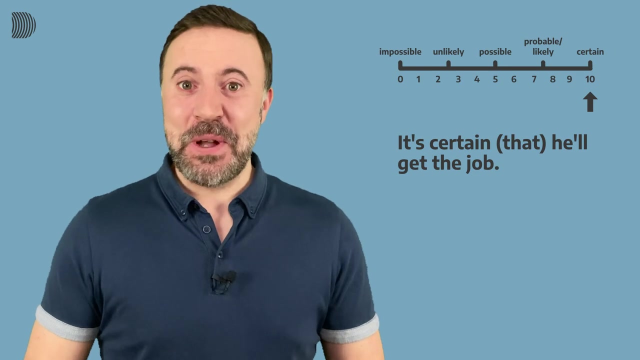 the job. and for the last of these simple example sentences, we'll imagine that michael is the only person who was invited for an interview and that the company really wants to hire him. so we can say it's certain he'll get the job. say it with me, it's certain he'll get the job. okay, so those were some. 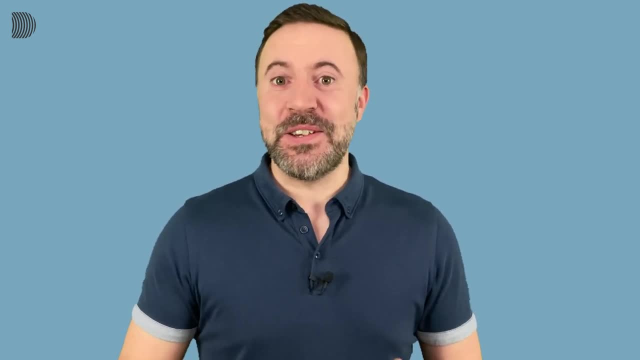 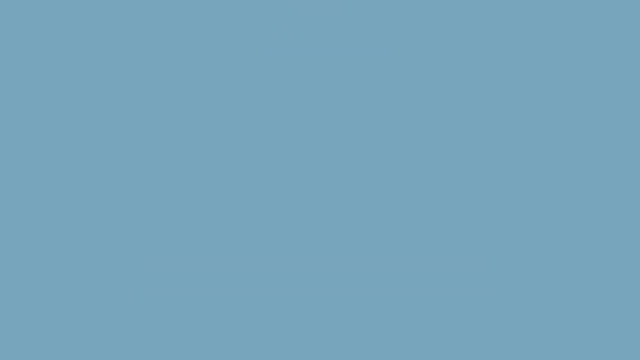 very simple example sentences to express degrees of certainty about the future. now let's look at some other possibilities to talk about michael and this job. let's remind ourselves of the very important thing about him. one thing about michael: that's jaguar tells everyone that he is certain. 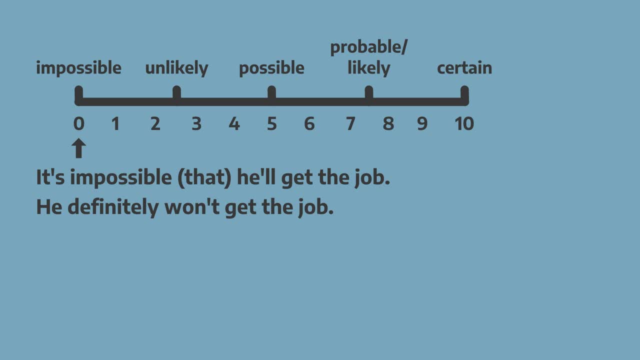 he's getting him to minimum a job now. you would always have to think about this one, not only when you talk about him between men, but the difference between a man and a woman. explain this to everyone. to explain he's getting a job. he's bathroom card exam at the end of the day, but 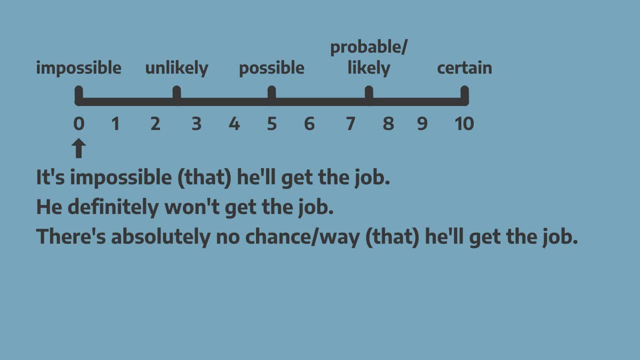 it is astonishing that there is no girl on the job list to explainать a job that's necessary was propagate. no way he'll get the job. one, two, three. there's absolutely no way he'll get the job, or the chances he'll get the job are zero. one, two, three, the chances he'll get. 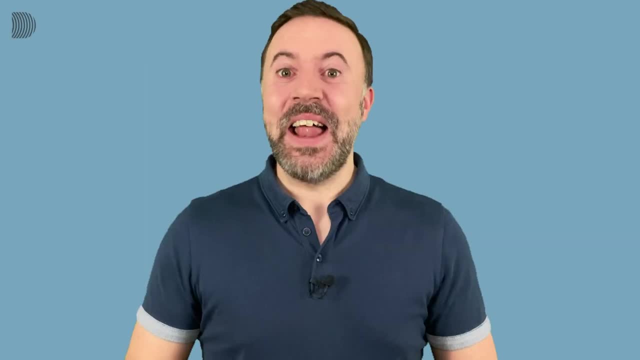 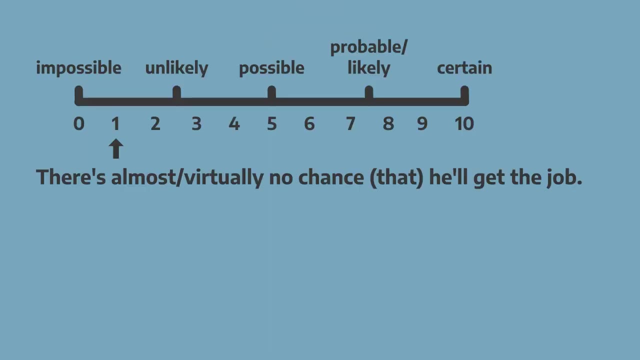 the job are zero. and now let's take a look at some examples. for number one on the scale, there's almost no chance he'll get the job. one, two, three, there's almost no chance he'll get the job. or there's virtually no chance he'll get the job. 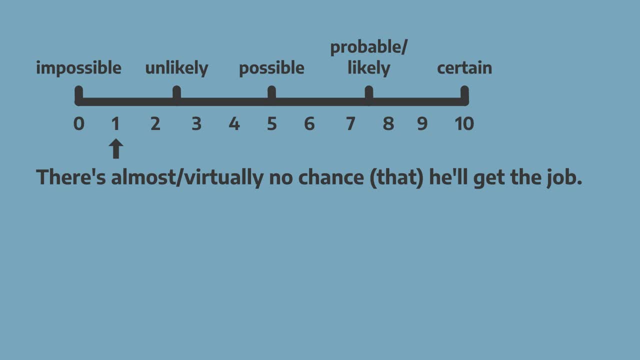 one, two, three. there's virtually no chance he'll get the job. almost and virtually have the same meaning here. it's very unlikely he'll get the job one, two, three. it's very unlikely likely he'll get the job or it's highly unlikely he'll get the job one, two, three. 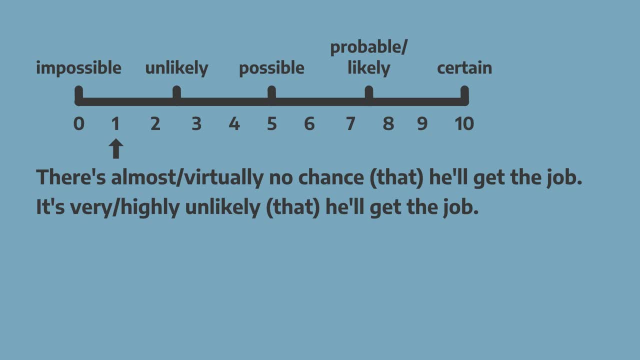 it's highly unlikely he'll get the job, or the likelihood he'll get the job is very low. one, two, three. the likelihood he'll get the job is very low, or the chances he'll get the job are very low. one, two, three. the chances he'll get the 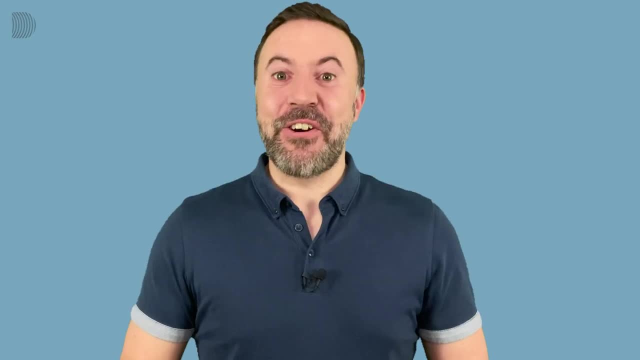 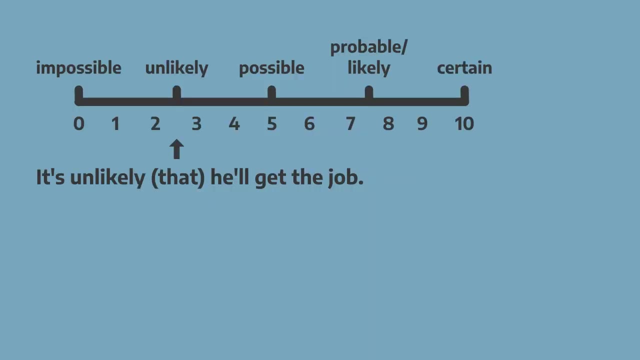 job are very low, great. and now let's move on to the next part of the scale and remind ourselves of our first example sentence: it's unlikely he'll get the job. it's unlikely he'll get the job, or there's a small chance he'll get the. 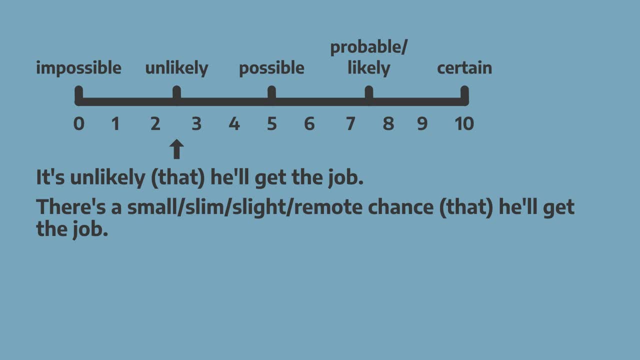 job- one, two, three. there's a small chance he'll get the job. or there's a slim chance he'll get the job- one, two, three. there's a slim chance he'll get the job. or there's a slight chance he'll get the job- one, two, three. there's a slight. 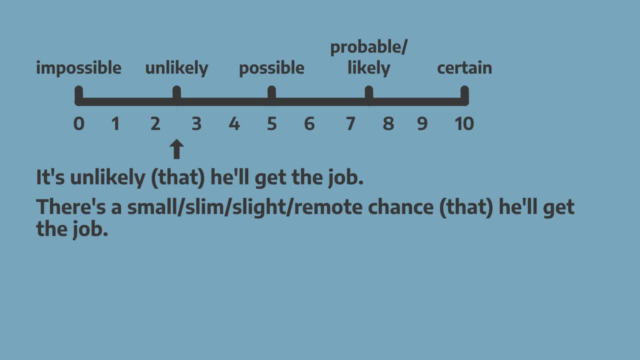 chance he'll get the job, or there's a remote chance he'll get the job. one, two, three: there's a remote chance he'll get the job. so all four words here have the same meaning: small, slim, slight and remote. they all represent a very small chance. and one more example: he probably won't. 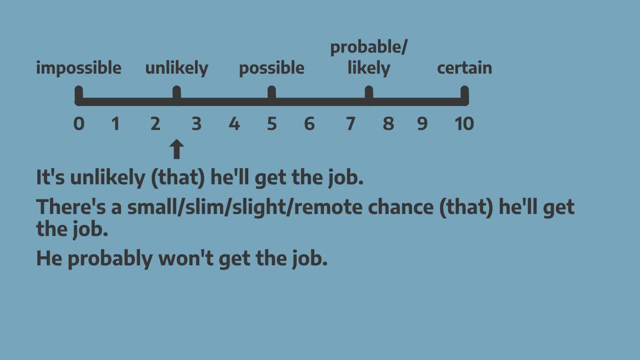 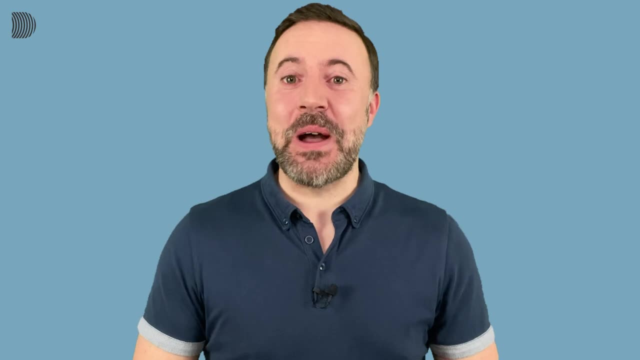 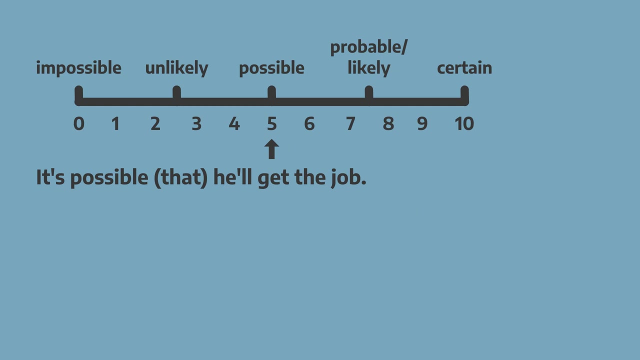 get the job. one, two, three, he probably won't get the job. and now let's take a look at some different ways to talk about the middle of the scale and we'll remind ourselves of our first example. it's possible he'll get the job, it's. 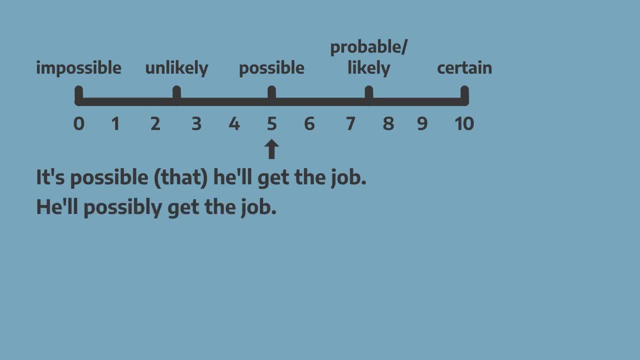 possible he'll get the job. or he'll possibly get the job one, two, three. he'll possibly get the job. or there's a possibility he'll get the job. one, two, three. there's a possibility he'll get the job. so we skipped number four. for this part of the scale we could say something like there's a slight 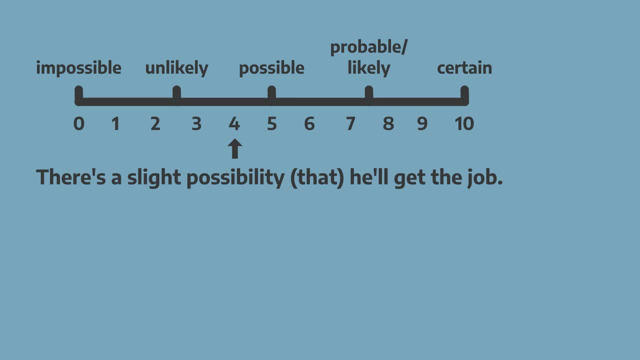 possibility he'll get the job. one, two, three. he'll get the job. one, two, three. there's a slight possibility he'll get the job. and if we say there's a strong possibility he'll get the job, it's between six and seven. repeat after three: one, two, three. there's a strong possibility he'll get the job. 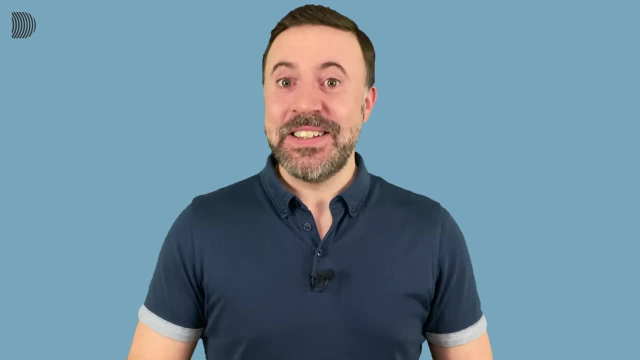 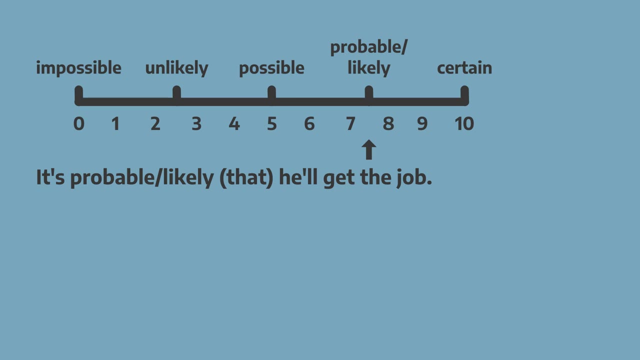 excellent. and now on to the next part of the scale, seven to eight, and our first example was: it's probable or it's likely he'll get the job. it's probable or it's likely he'll get the job or he'll probably get the job. one, two, three, he'll. 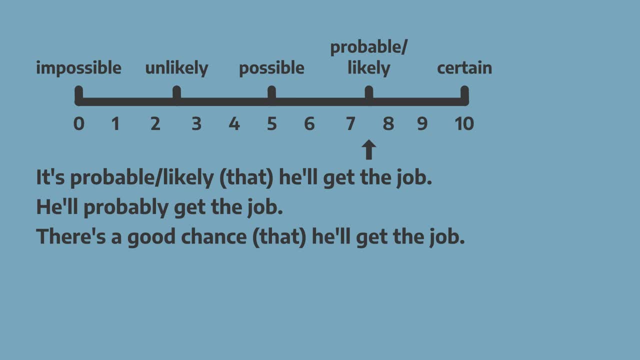 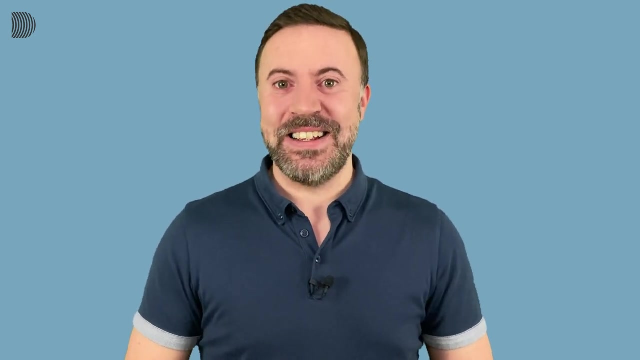 probably get the job, or there's a good chance he'll get the job. one, two, three. there's a good chance he'll get the job. great, and now let's take a look at some different ways to define a bad sentence. talk about number 9 on the scale. There's almost no doubt he'll get the job. 1,, 2,, 3.. There's almost 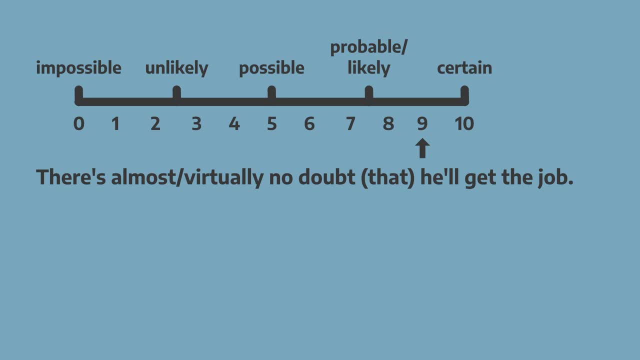 no doubt he'll get the job. If there is no doubt about something, it means it's very certain, very sure. Be careful with the pronunciation of this word. The B is silent, Doubt, Doubt. Moving on to the next example, It's almost certain he'll get the job. 1,, 2,, 3.. It's almost. 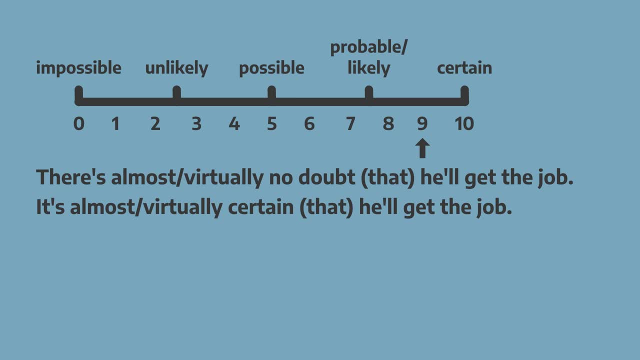 certain he'll get the job Or it's virtually certain he'll get the job. 1,, 2,, 3.. It's virtually certain he'll get the job Or the likelihood he'll get the job is very high- 1,, 2,, 3.. The 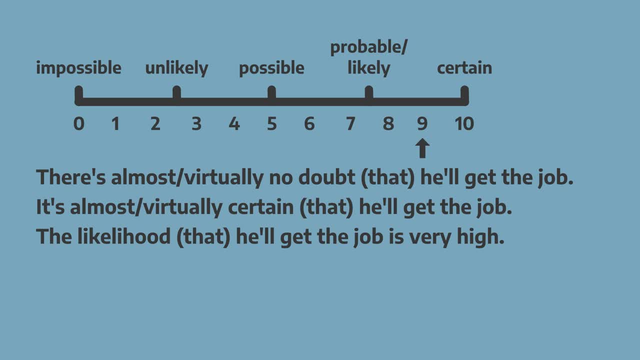 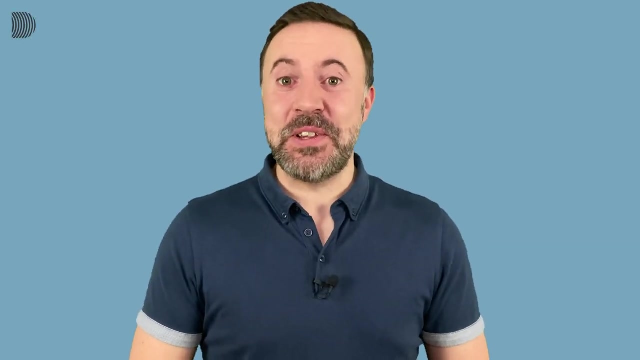 likelihood he'll get the job is very high. and one more example: the chances he'll get the job are very high. one, two, three: the chances he'll get the job are very high. and finally, we'll take a look at some different ways to talk about the. 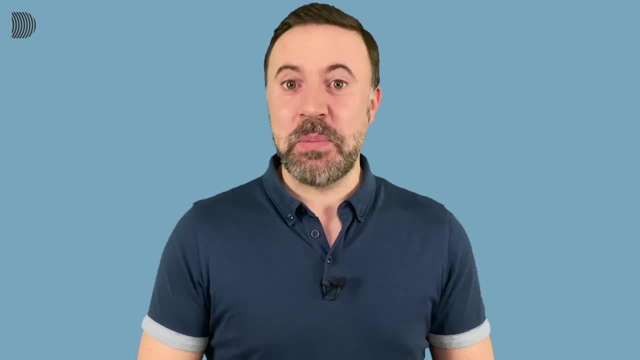 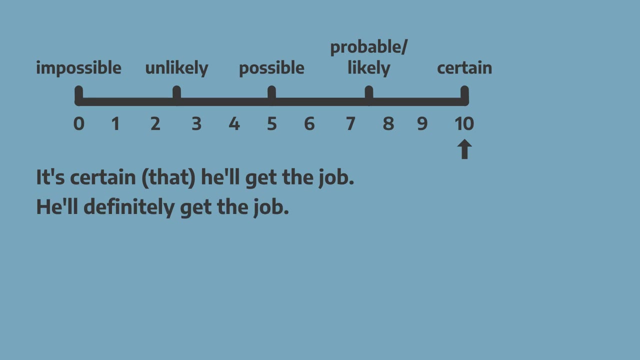 highest end of the scale. if you remember our example: it's certain he'll get the job. it's certain he'll get the job, or he'll definitely get the job. one, two, three, he'll definitely get the job. and our final example: there's absolutely no doubt he'll get the job. 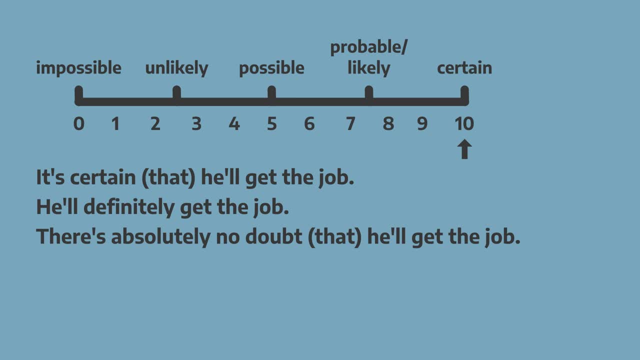 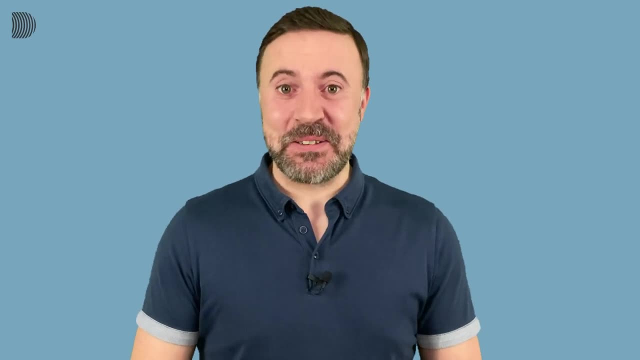 one, two, three. there's absolutely no doubt he'll get the job great. and now it's time for our quiz. you'll see six sentences and for each one you'll have to decide which number on the scale it applies to. you have three seconds for each sentence. good luck. 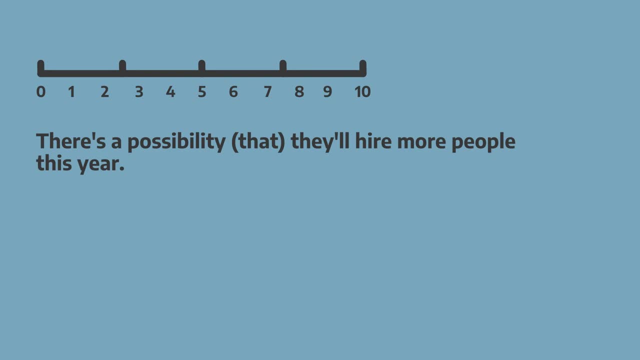 there's a possibility they'll hire more people this year. this new product will definitely help to increase sales. there's virtually no doubt the company will lose money this year. there's a slight chance turnover will increase in the next two weeks. it's highly unlikely. susan will finish the report today. 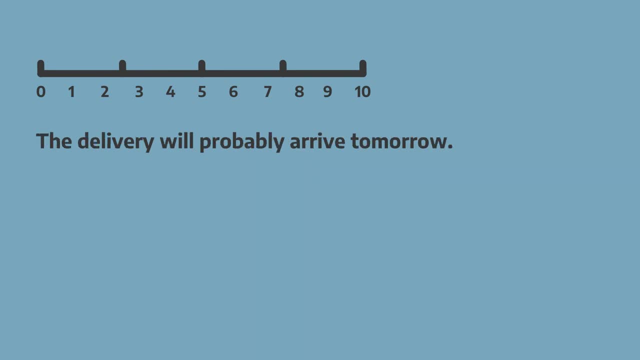 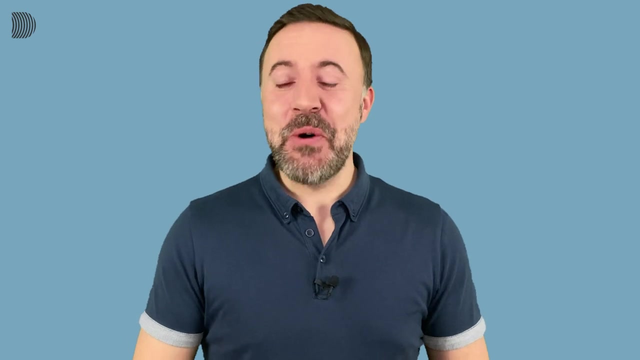 the delivery will probably arrive tomorrow. and how did you do on the quiz? hopefully you did well and hopefully you like this lesson. all of the examples are included in the description below. why not try your own example sentence? write it in the comments and i'll give you some feedback and i'll see you in the next.